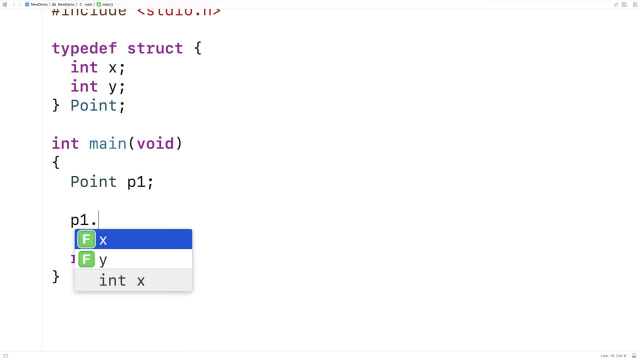 member variables. we're going to use the dot notation. So I'll say p1 dot x is equal to 3 and p1 dot y is equal to 3.. So I'll say p1 dot x is equal to 3 and p1 dot y is equal to 3.. 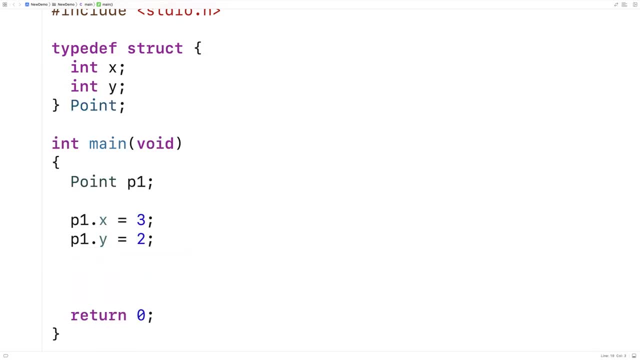 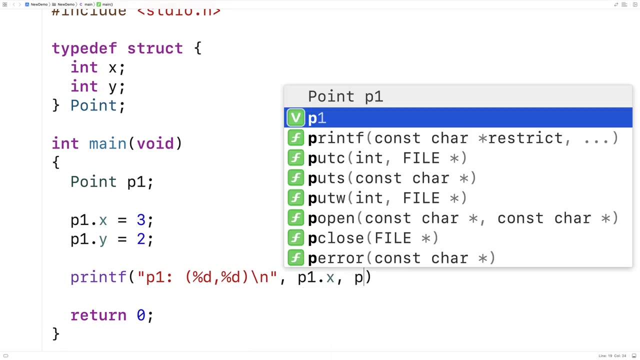 This is how we can access and assign to those member variables. We can use them expressions or function calls as well. So here I'll say: printf: p1 percent d, comma percent d slash n, and we'll output p1 dot x and p1 dot y, and if I save this here and run it, we'll get the expected tuple here. 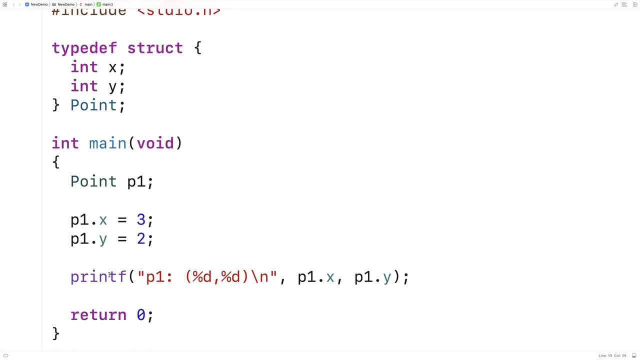 as output 3 and 2.. So this is working with a regular struct variable. What if I have a pointer to a struct? So here I'll say point star p2, and what I have here now is a pointer to a struct. So it's going. 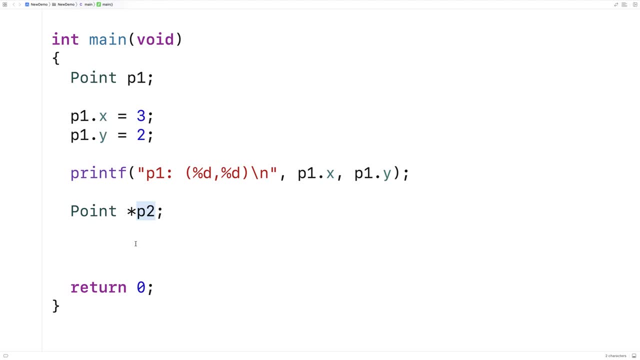 to store the memory address of a struct, I'd have to assign to it the memory address of an existing struct or dynamically allocate space for a struct in order to actually access member variables through this pointer here. So let's do the first thing, Let's actually assign to p2 the memory. 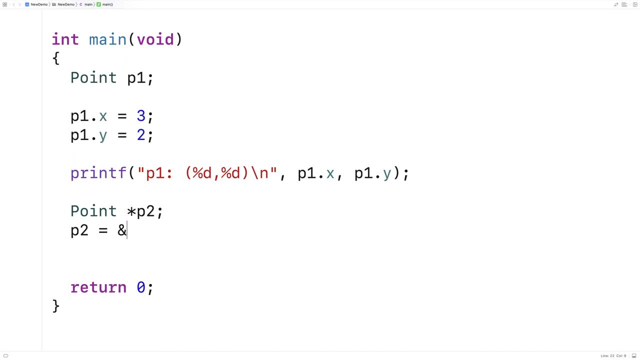 address of p1.. So here I'll say p2 is equal to and p1.. So right now p2, we would say, is pointing to p1, and I could actually access the member variables of the struct now with the arrow notation. So I could say here: p2, dash x, is equal to, let's say, 5. now 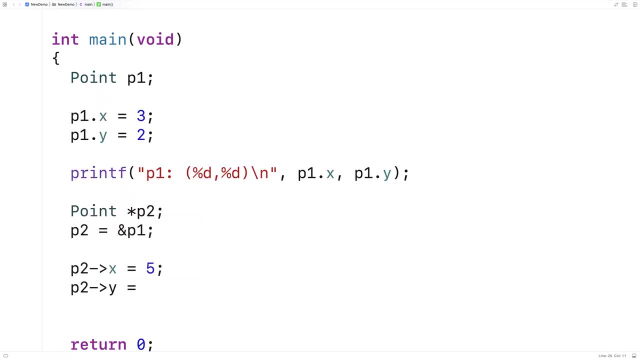 and p2 dash y is equal to maybe 4 now, and what I'm doing here is I'm actually changing the member variables x and y of whatever p2 is pointing to, and so in this case here it's p1, assigned to it the memory address of p1.. So now, if I go to output p1, I'll find that it's actually 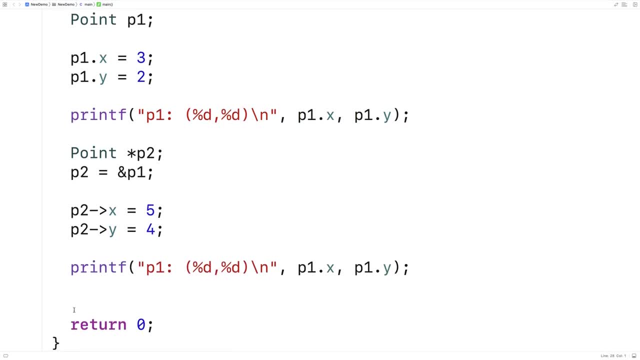 been set to these values here: 5 and 4.. So I save this here now and run it, and we should get that p1. the second time it's printed is 5 and 4, and we do Now. we could also access these member. 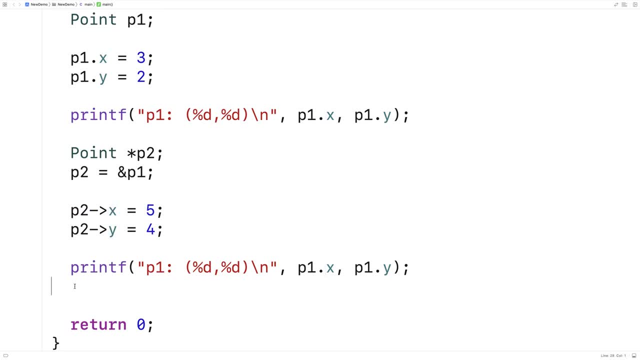 variables here, x and y, via p2.. So I could say here printf, and we could say maybe p2, and I'll say p2 arrow x, p2 arrow y, and if I save this here and run it, we're going to find these are the same. 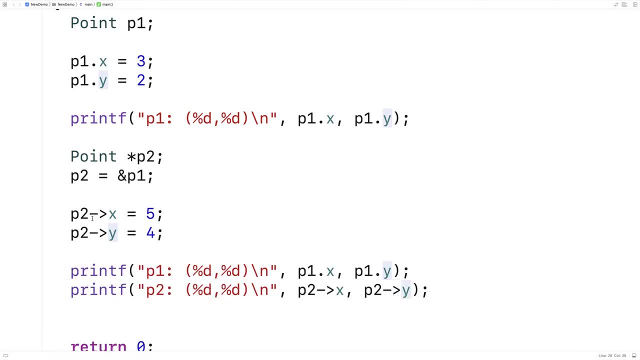 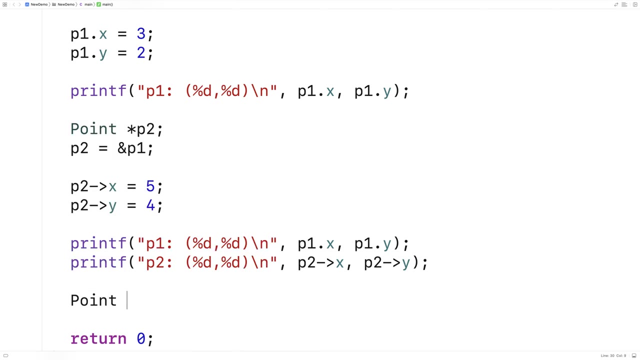 thing. So this arrow notation. it gives us access to the member variables of the struct that this pointer to a struct, in this case point, is pointing to. So we could do some more stuff here. Let's make a pointer and we'll allocate space dynamically for the struct. So here I'll say: point star, p3. 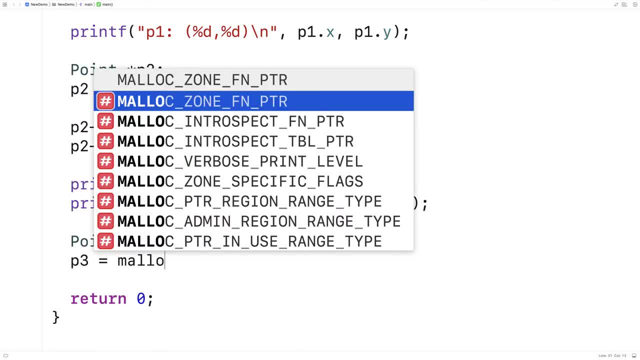 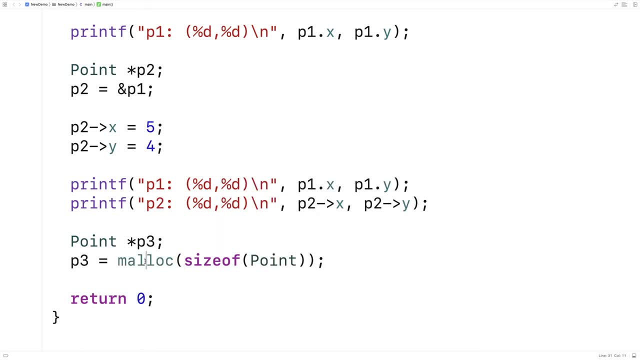 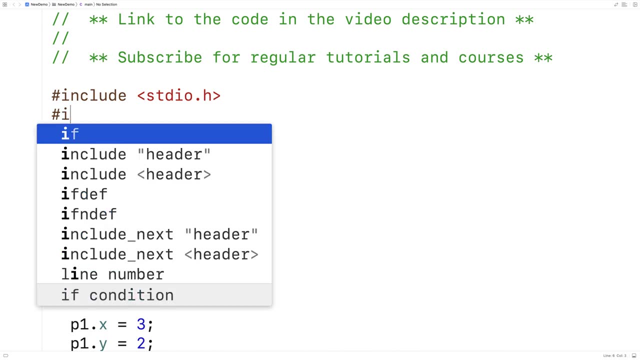 and I'll say p3 is equal to malloc size of point. So because I'm using the function malloc, I'm going to have to include the stdlibh library. This function allows me to dynamically allocate space for things, including structs, and we have to include stdlibh if we're going to use it, because that's where the 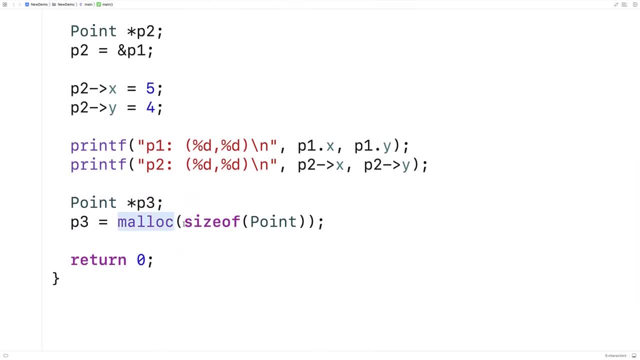 function is defined And here we're saying: go, get enough space to store something as large as a point. So size of point returns how many bytes are needed to store a point. So this will actually return a memory address for a block of memory large enough to store a point. 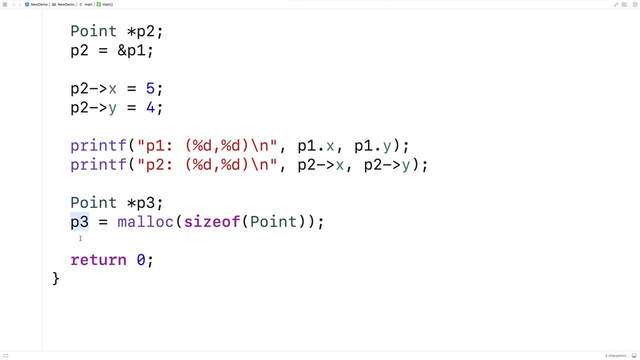 and p3 is going to contain that memory address. It's going to point to this dynamically allocated space. So now I can actually access the member variables of p3 using the arrow notation as well. So I could say: p3- x is equal to 5, p3- y is equal to 10, and then we can output p3 with similar code. 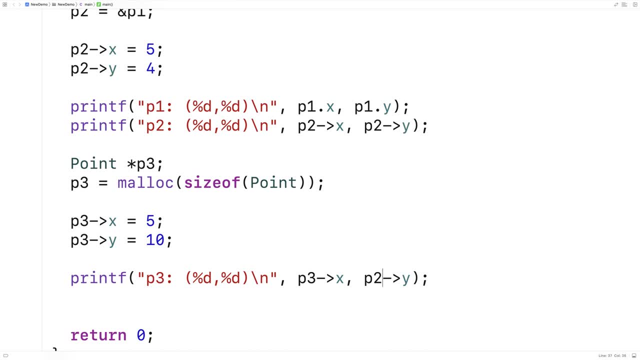 say p3, p3 x, p3 y. if we save this and run it, we expect that p3 should be 5 and 10.. So this arrow notation basically saves us from having to use something like the dereference operator, because another way I could get at these member variables is with the dereference operator, followed by the. 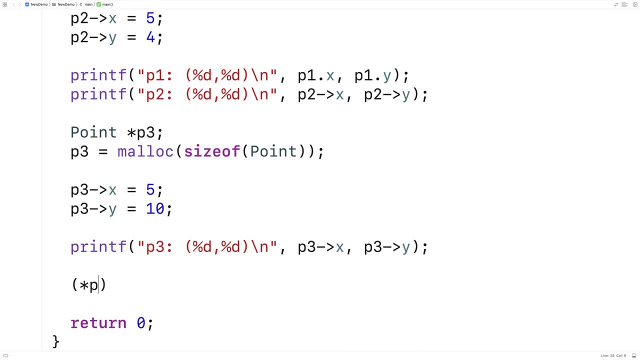 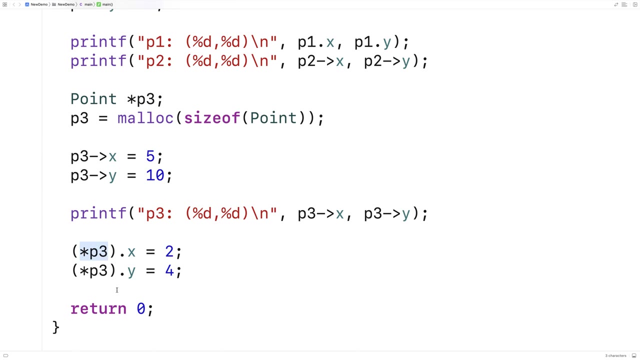 dot operator. So I could say, for example, star p3 dot x is equal to 2 and star p3 dot y is equal to 5, and this will actually work as well. What the dereference operator does is it goes and gets whatever the pointer is pointing to. So in this case, here it's going to go and get what's actually. 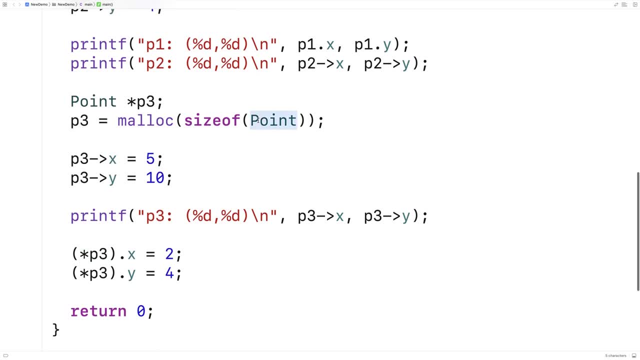 pointed to by p3, which is this point: struct here, and then, once we've got that, we can actually just use the dot notation. We do have to put these brackets, though, around the dereference operator. because of the order of operations, We have to make sure that this dereference operator happens. 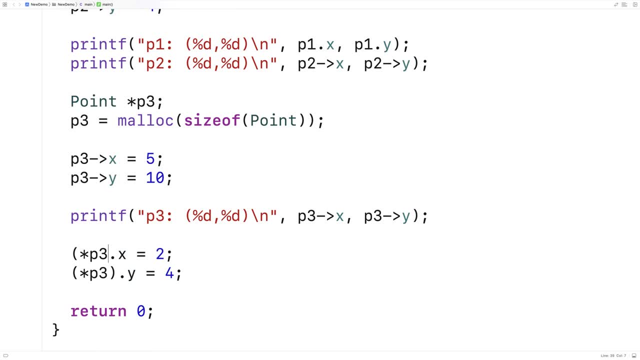 first before we attempt to use the dot operator. If we don't have the brackets, it'll actually not work. So if I save this here and try to run it, it's going to complain here. If I put the brackets around it, though, we're good. and what's happening? 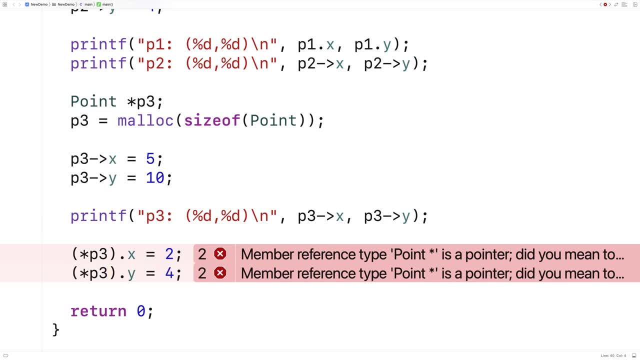 is the dereference operator is happening: first We're going and getting what p3 is pointing to, in this case a point- and then we're using the dot operator to actually access the values that are at that struct. So we could output p3 in a similar way. here I could say star. 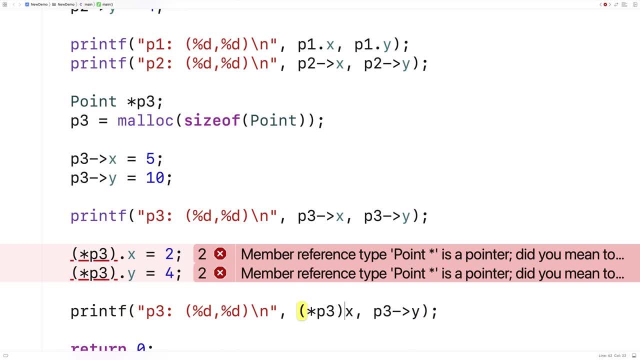 p3 dot x is equal to 2 and star p3 dot y is equal to 2 and star p3 dot y is equal to 2.. And if I save this here and run it, we'll get that p3 is now going to be 2 and 4 here. 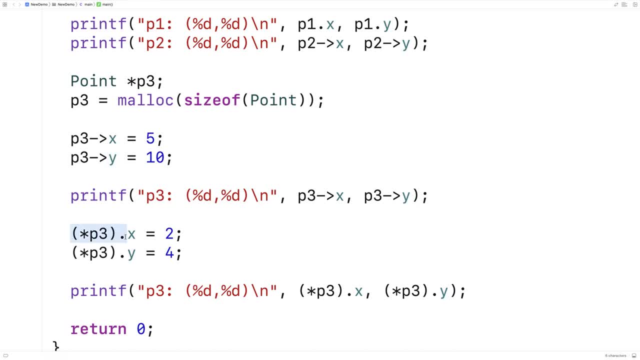 So this notation here of using the dereference operator followed by the dot, it's kind of ugly. You might forget to put the brackets. It's not very nice to look at. This error operator seems to make a lot more sense, It's a lot more direct, and so they give us the error operator in c. 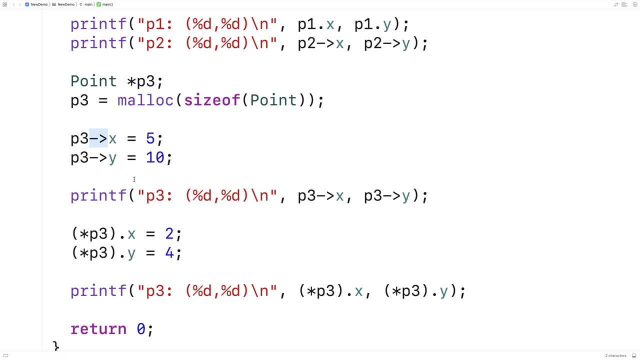 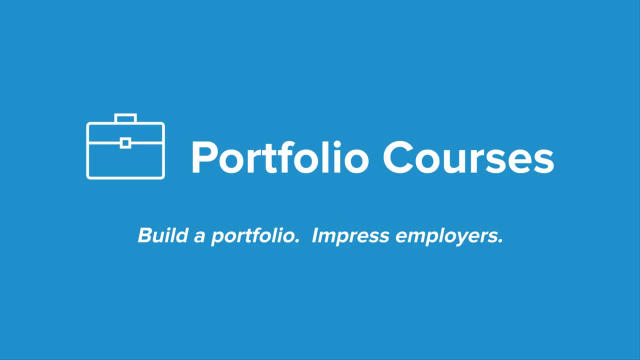 So this is how you can use the error operator to access the members of a struct. when you have a pointer to the struct in c, Visit PortfolioCoursescom, where we'll help you build a portfolio that will impress employers, including courses to help you develop c programming projects.